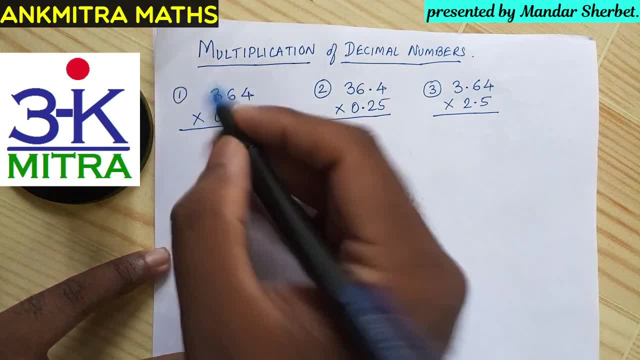 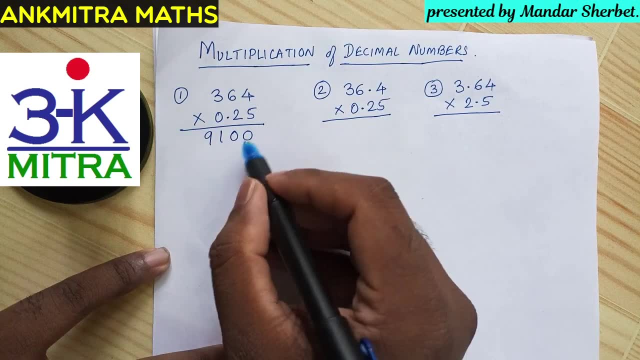 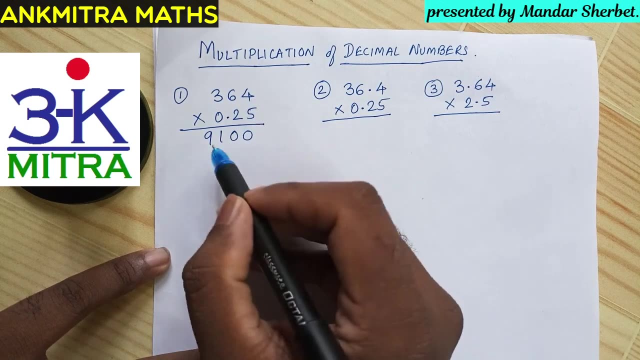 to write down the number of digits and then the answer that we get is 9100.. So 9100 is the answer after multiplying 364 by 25.. Remember, this is not the final answer. Now for the final answer what the second step we have to do, which is to place the decimal point at the appropriate. 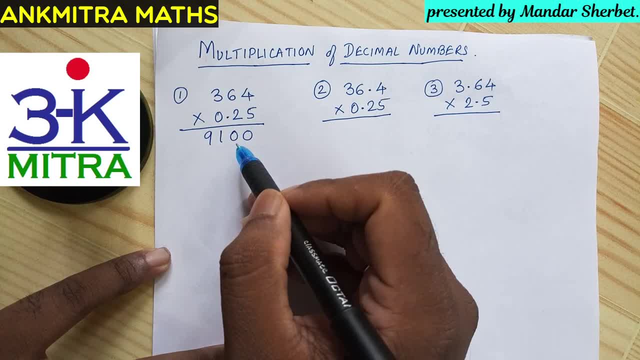 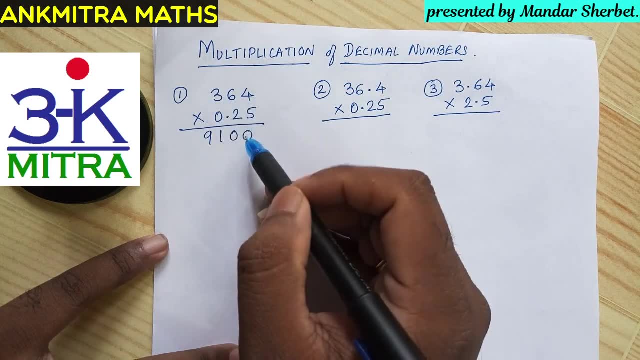 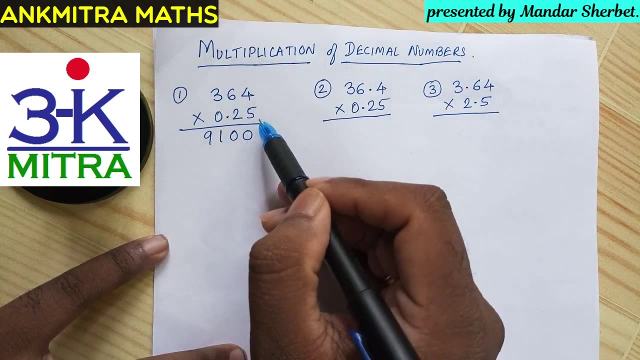 location. So which is the appropriate location? So how do you find that is? first count the number of digits after the decimal point in both the numbers. in the first number it is 364 completely. There is no decimal point here. In the second number it is 0.25. so there are. 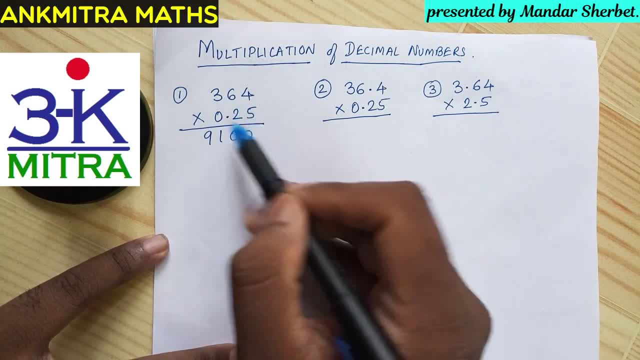 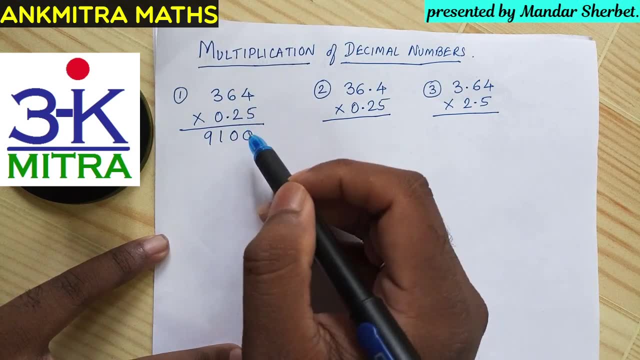 two digits after the decimal point. So the total number of digits after the decimal point in both these numbers is just 2.. Okay, there are two digits after the decimal point in both these numbers. So in the final answer also the last two digits will will be after: 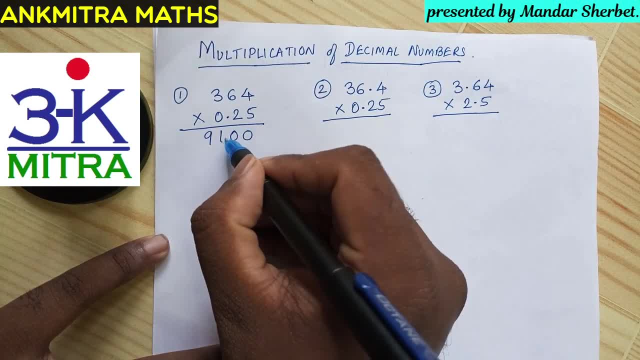 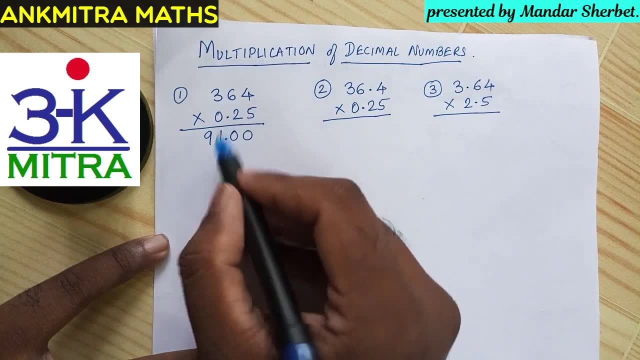 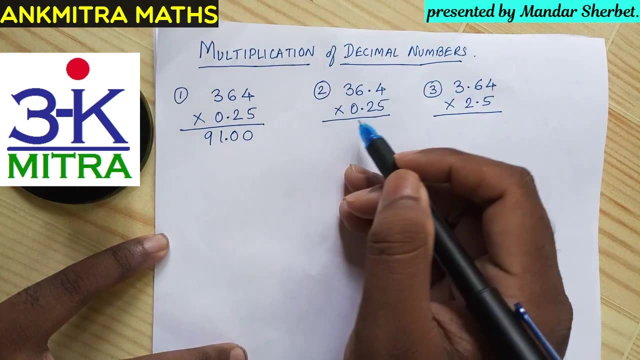 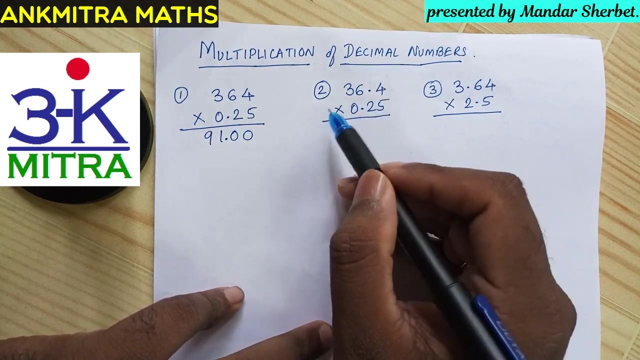 the decimal point. hence the appropriate location for the decimal point will be this: okay, so the final answer that we get for 364 multiplied by 0.25 is 91.00 or just 91. coming to the second sum, those rules are the same. so we'll first multiply 364 by 25 by ignoring any decimal point in both. 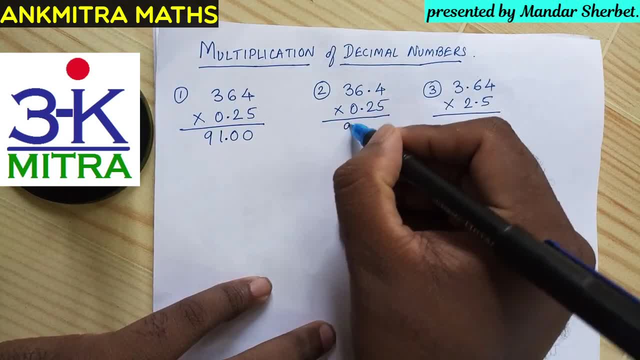 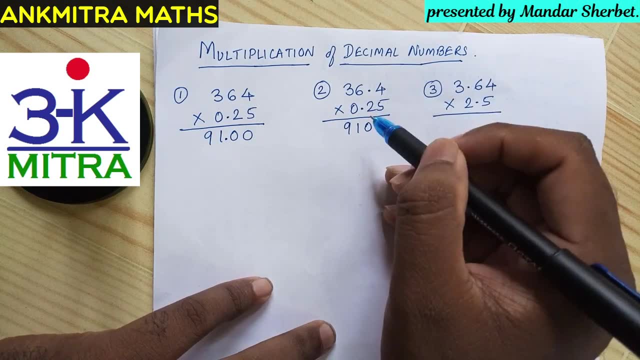 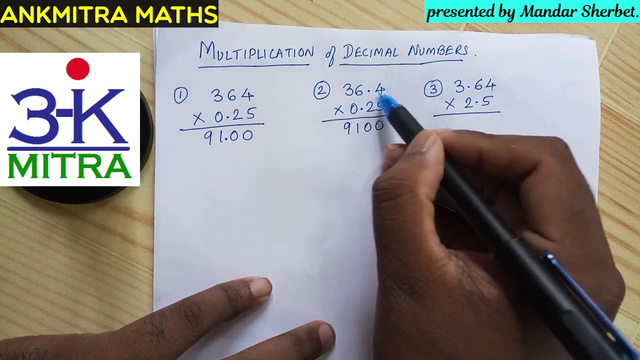 the numbers. so the answer that we'll again get is 91.00. now for the second step, that is, to arrive at the final answer. we have to count the total number of digits that we have after the decimal point in both these numbers. so in the first number we have one digit after the decimal point, that is. 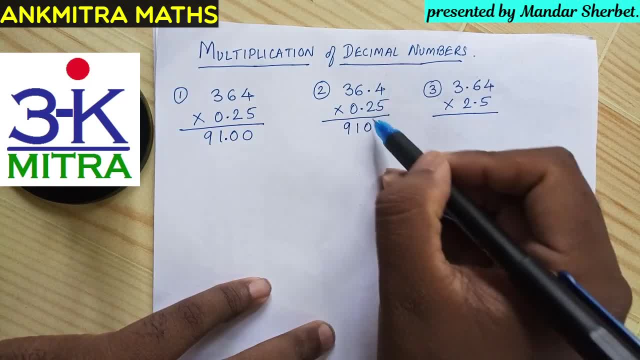 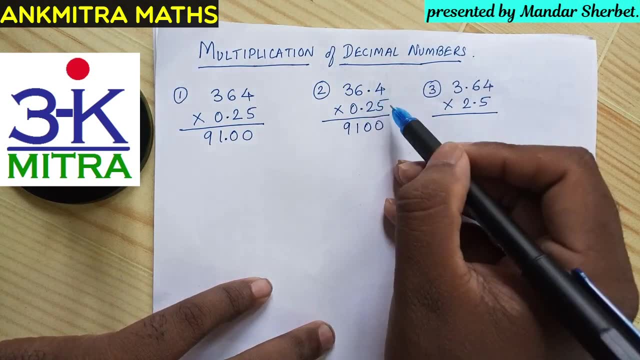 36.4. we have one digit after the decimal point in this number. we have two digits after the decimal point. hence the total number of digits after the decimal point in both the decimal points. these numbers is three this time. okay, we have three digits after the decimal point in both. 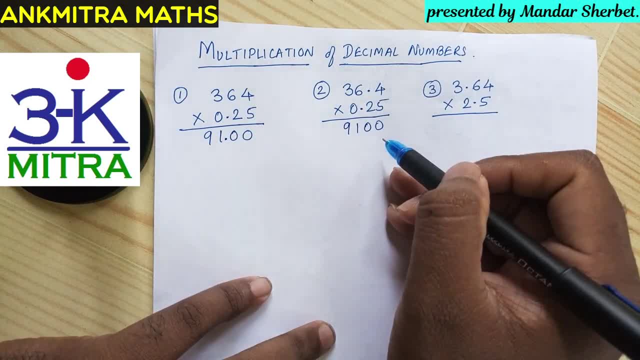 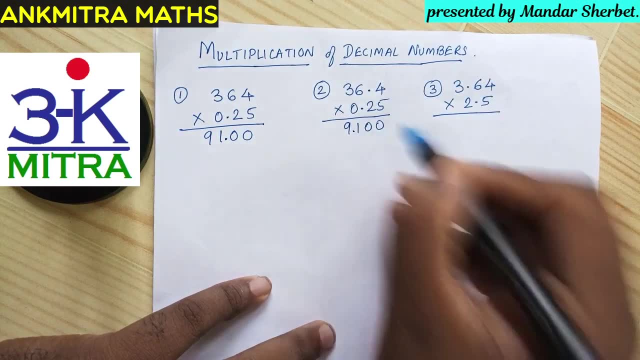 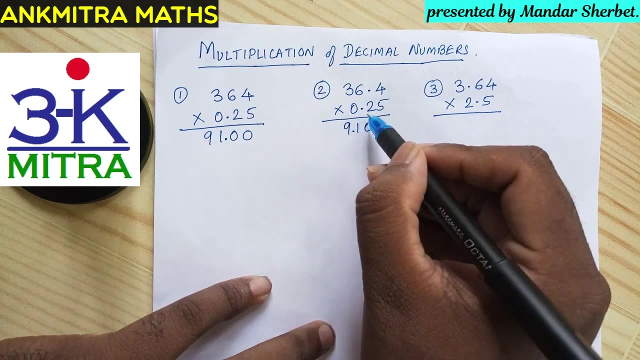 these numbers. so in the final answer we will have to place a decimal point in such a fashion that there will be three digits after the decimal point. so the decimal point will be here, leaving the last three digits after it. okay, so the final answer for 36.4 multiplied by 0.25 will be 9.1 or 9.100. okay, 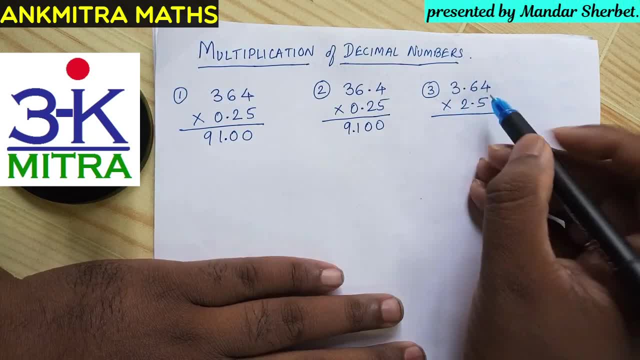 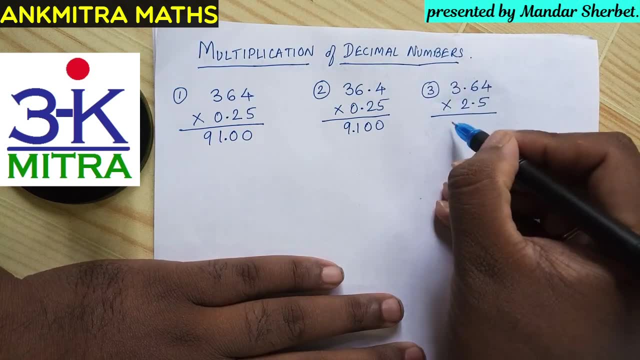 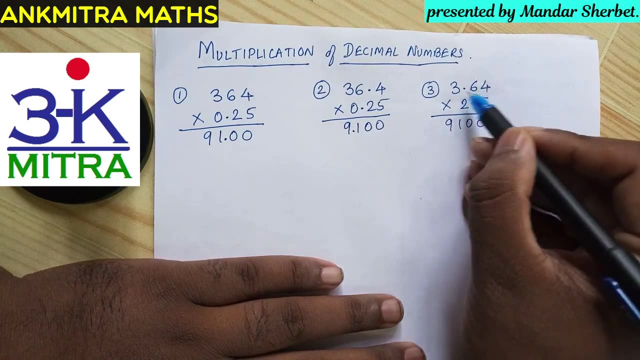 so we'll just read it. coming to the third example, it is again. first step to be done is multiply 364 by 25, ignoring the decimal points, and we get 9.1.0.0 again. now count the total number of digits after the decimal point. we have two digits in the first number after the decimal point, one digit in the. 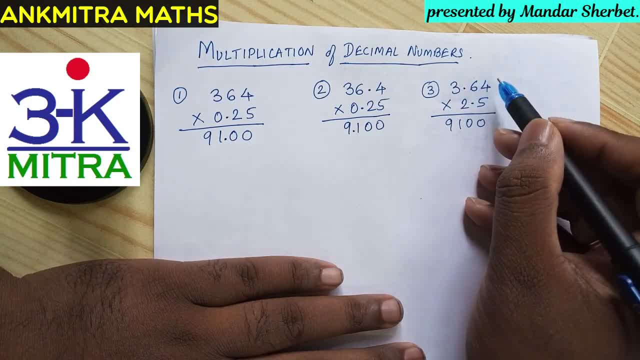 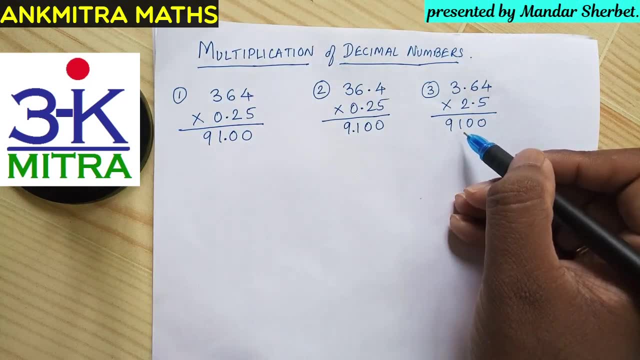 after the decimal point in the second number. so the total number of digits after the decimal point here again are three. so in the final answer also we will have three digits after the decimal point. we will have three digits after the decimal point, hence the appropriate location for decimal point. 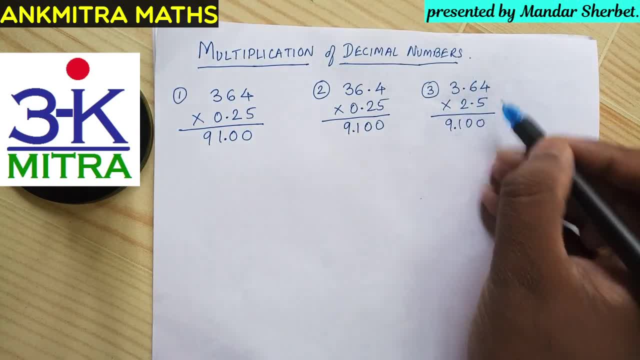 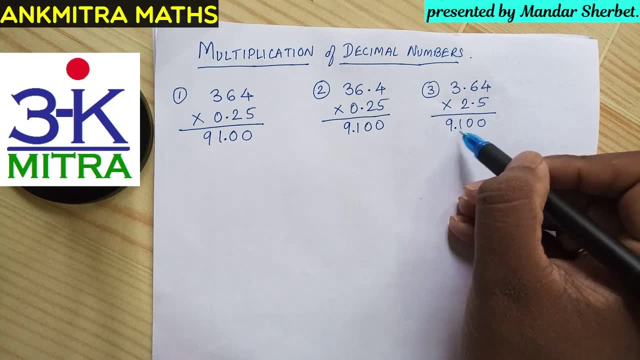 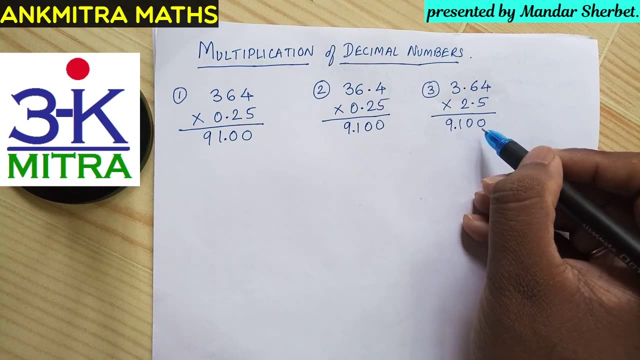 will be this: and the answer that we have for 3.64 multiplied by 2.5 is 9.1. again, okay, we can read it as 9.1 or we can read it as 9.100, doesn't matter. the last two digits, these two zeros after the. 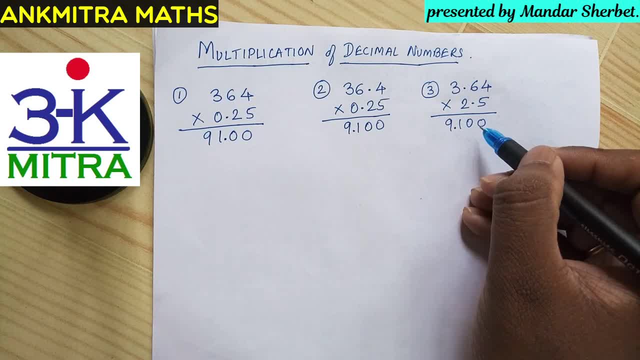 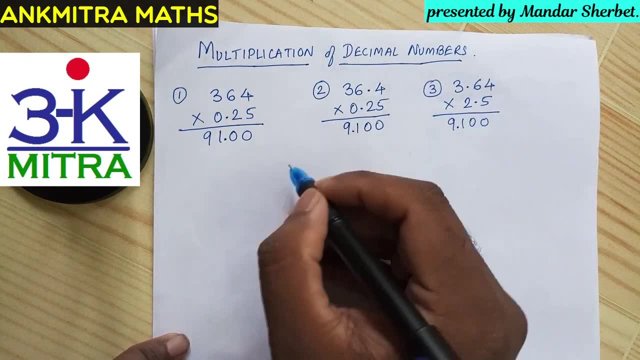 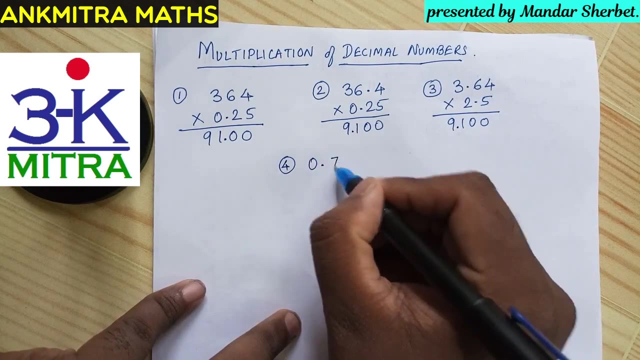 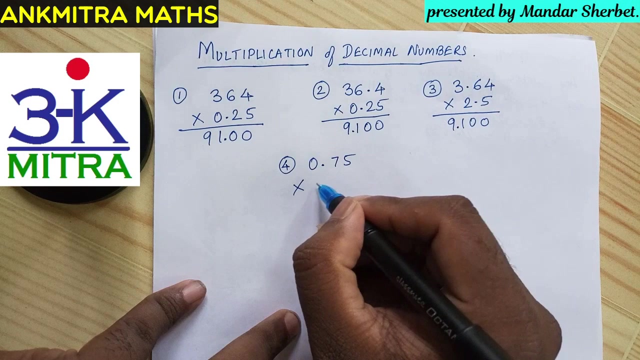 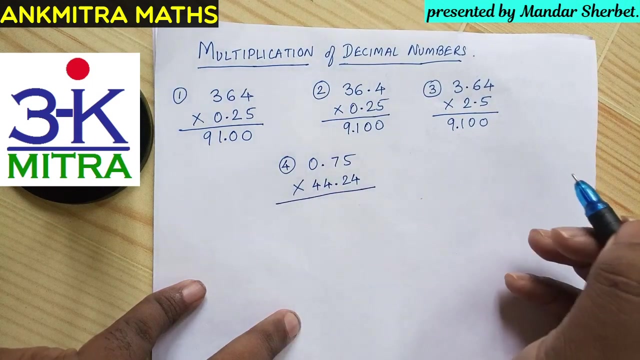 decimal point. the end zeros do not matter, even if you read them or not. let's take one more example, in this case a random example. let's say we are supposed to multiply 0.75 multiplied by, let's say, 44.24. okay, so first we will have to multiply 75 with 4.4. 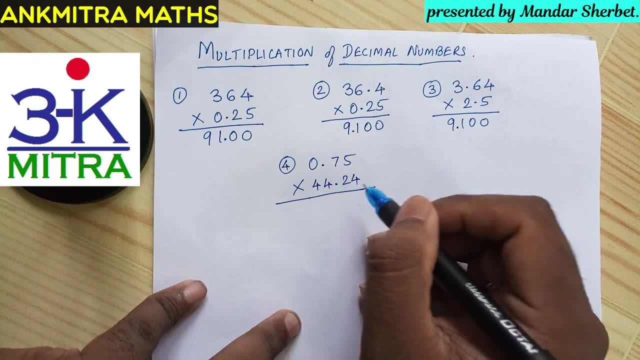 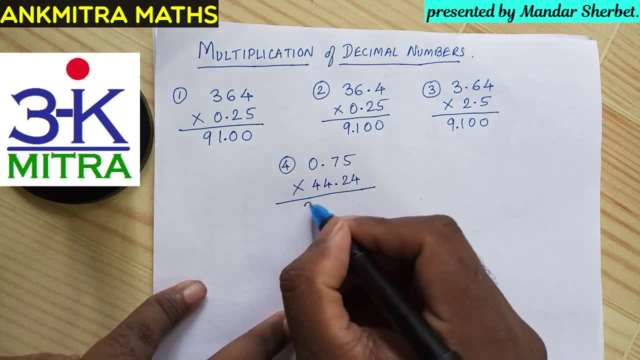 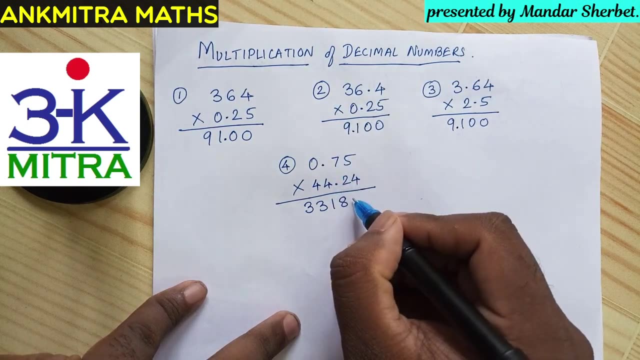 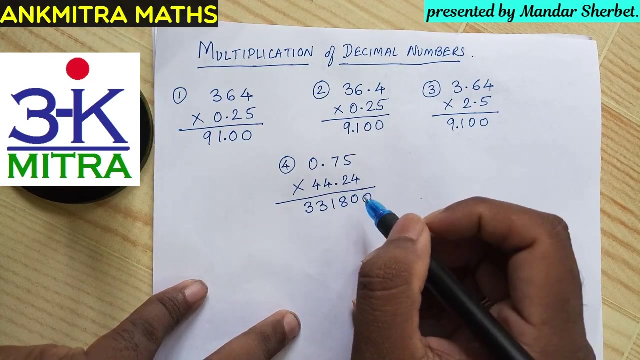 ignoring any decimal point here. so the answer that we get after multiplying 75 with 44.24 is: i think it should be 3, 3, 1, 8 and, uh, two zeros okay. so 3, 3, 1, 8, 0, 0 is the answer. i think that. 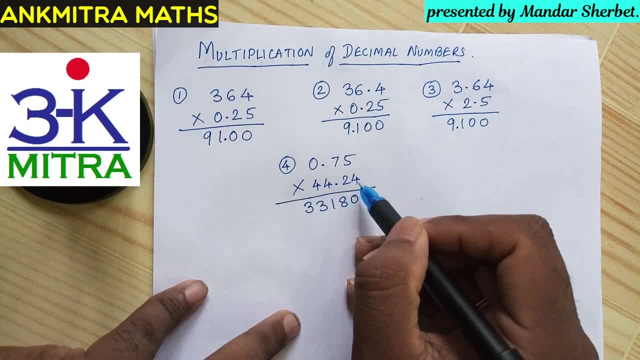 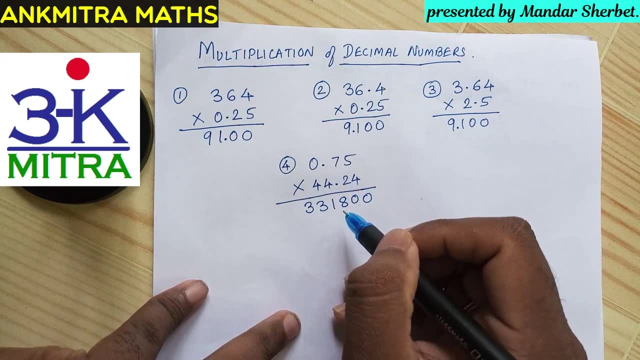 we'll get, after multiplying 75 with 4, 4, 2, 4 um. and now for the second step. we have to place the decimal point at the appropriate location. so first we'll count the total number of digits that we have after the decimal point in the given.